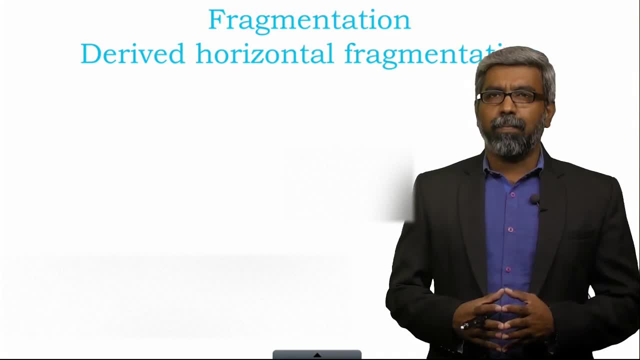 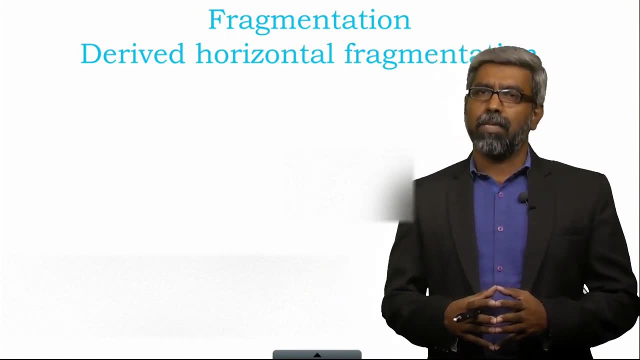 a relation. So when we fragment a relation, so we need a set of conditions, So we call it a simple predicate, So it is taken from the applications that are accessing the data at different sites. So each query: what are the conditions given in the WHERE class? These 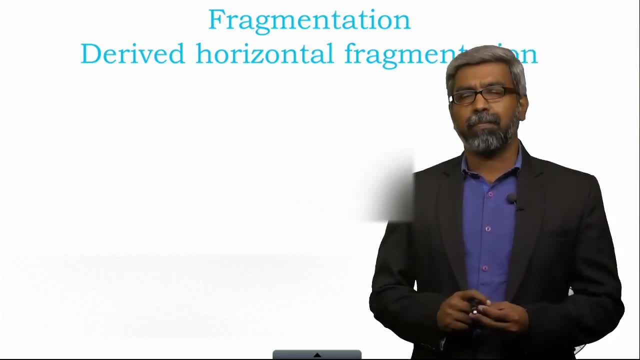 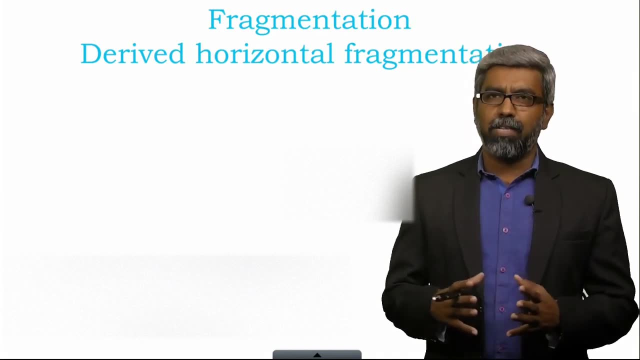 conditions could be used for deciding the simple predicates. So, after deciding the simple predicates, we need a set of conditions. So what are the conditions given in the WHERE class? These conditions could be used for deciding the simple predicates. So, after deciding the simple predicates, we have apply the conjunction. 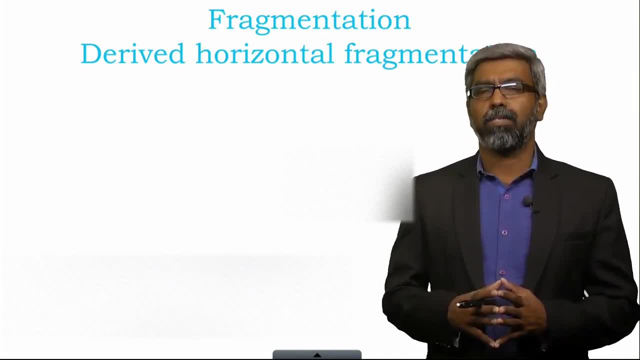 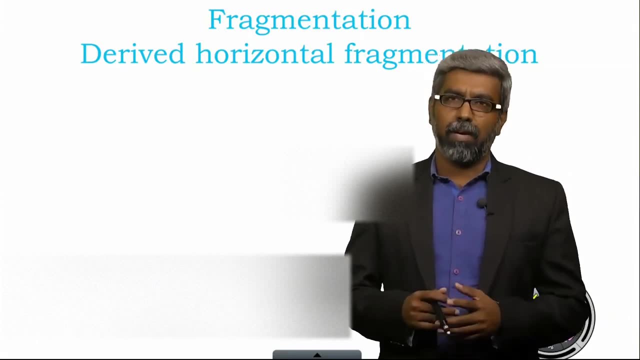 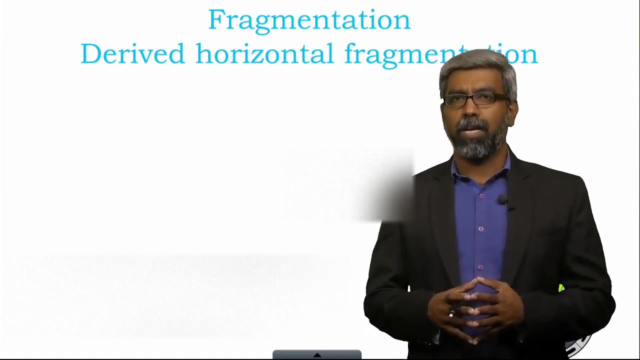 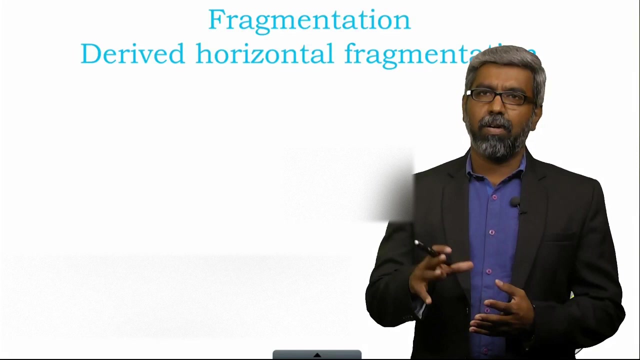 and negation of all these simple predicates to arrive at set of min term predicates. And these min term predicates were used to finally fragment a relation. And also we have discussed about the primary horizontal fragmentation. So primary horizontal fragmentation is basically a relation. R is taken and by applying a different 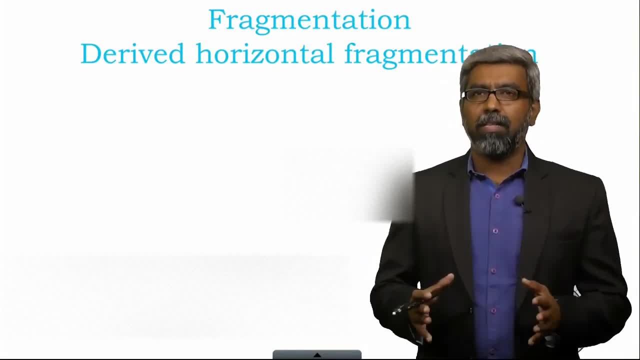 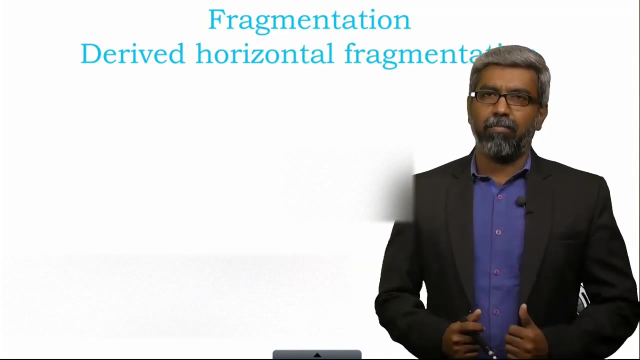 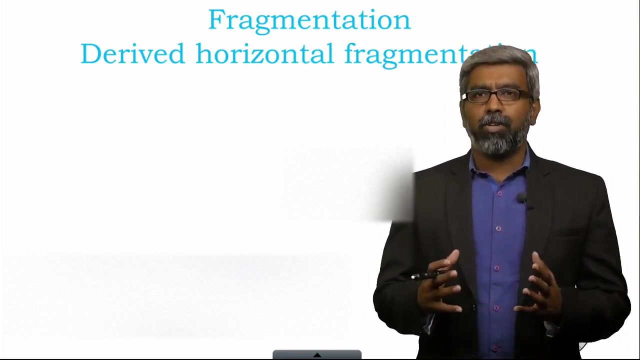 set of min term fragments. we are going to divide the table horizontally into several fragments So that we have used in the set of min term predicates to process to find the different set of min term fragments of the given relation. Now the question is: a database is collection of tables. It is not just one table, It is. 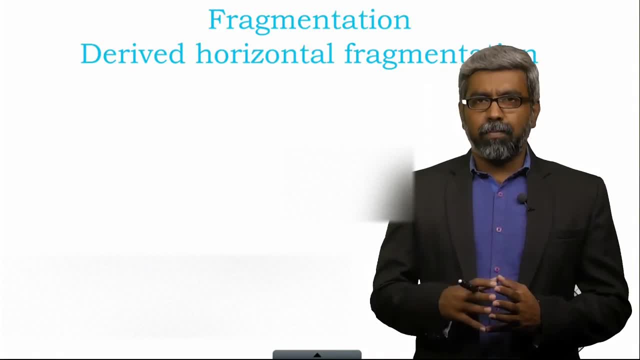 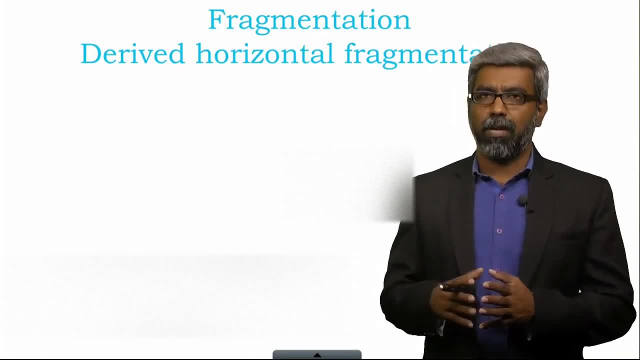 attribute is included in the another table as a foreign key, So it is going to refer. that is, the domain of these two are going to be same and we establish link between these two tables: the primary key and foreign key. Now the question is so when we derive, 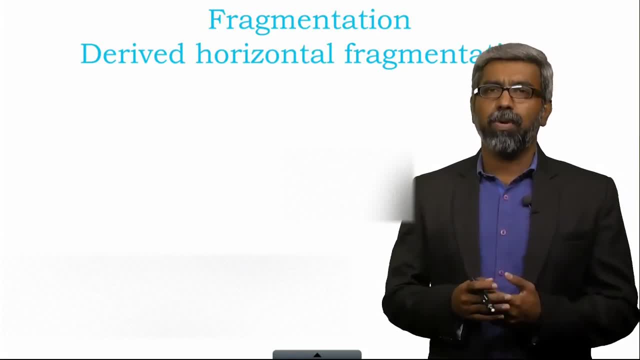 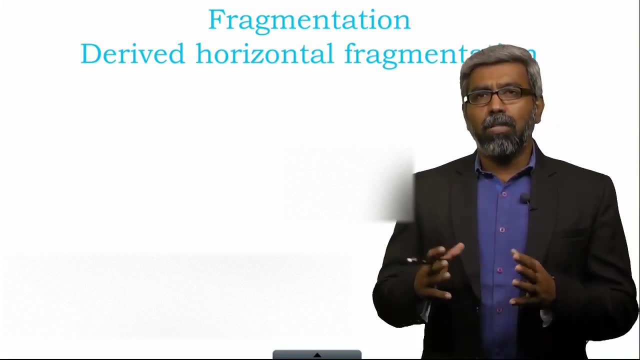 there is when we go for primary horizontal fragmentation. we consider just one table and in reality I cannot fragment all the individual tables using the set down table. So I cannot fragment all the individual tables using the set down table. So we have derived set of min term predicates. we have derived set of min term fragments. 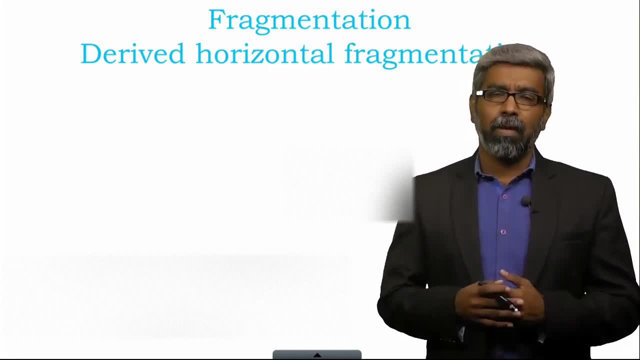 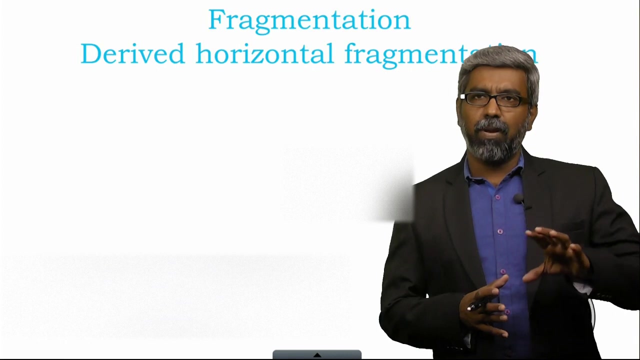 we have derived. It is a difficult task. The reason is, if I fragment one table on set of attribute, values on set of attribute, the same set of attributes may not present in other tables. Now the question is, how do we fragment the other tables? Because if we send, for example, a student, 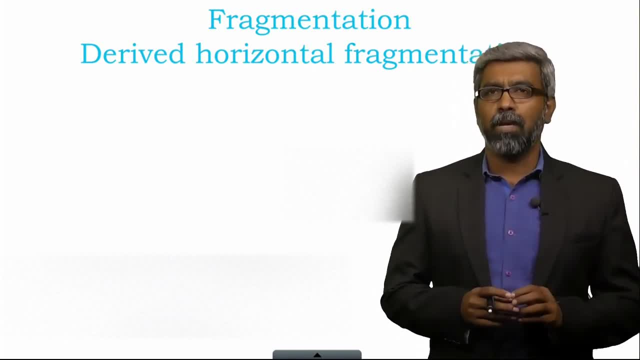 personal detail to one particular site and the mark details are stored in a different table and we must send the student mark detail to the same site. So how do we do that? So for that process we call this fragment as derived horizontal fragmentation. So the another. 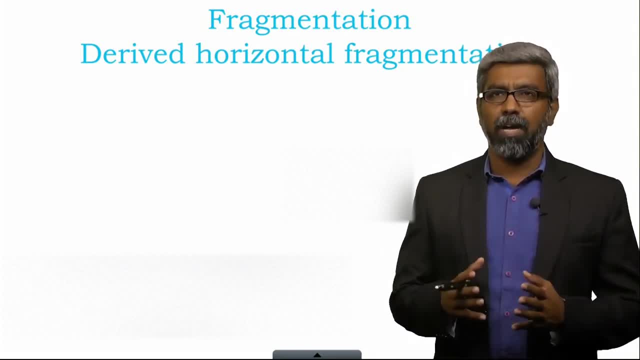 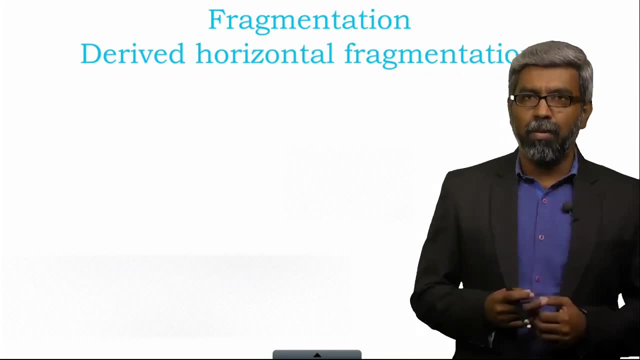 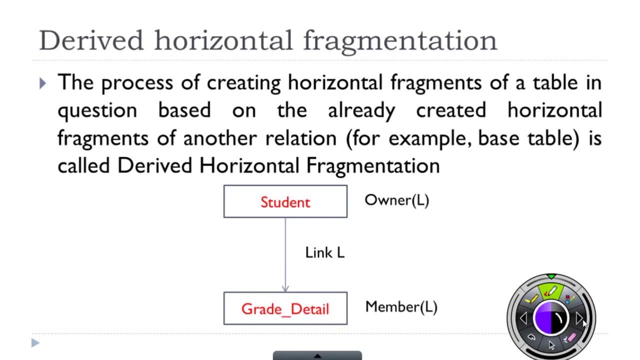 variety of horizontal fragmentation is derived horizontal fragmentation. Let us discuss about the derived horizontal fragmentation in this lecture. Now let us go to the presentation. Derived horizontal fragmentation is the process of creating the horizontal fragments of a table in Caustine based on the already. 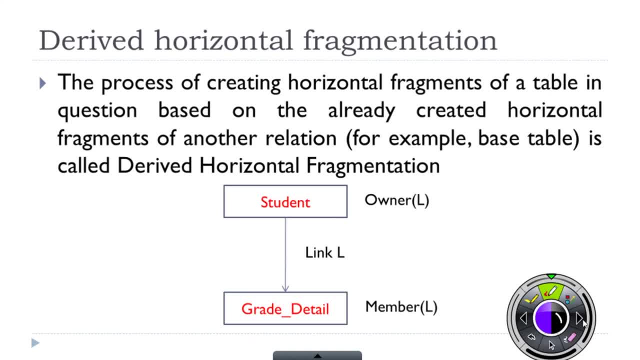 created horizontal fragment of another relation, For example the base table. This is called derived horizontal fragmentation. So when I have database, so relations, one relation is linked with other relation through the foreign key primary primary key, foreign key relationship. So we can, we may call that table with the primary. 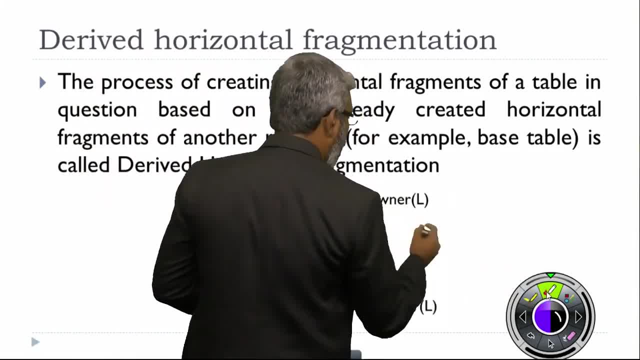 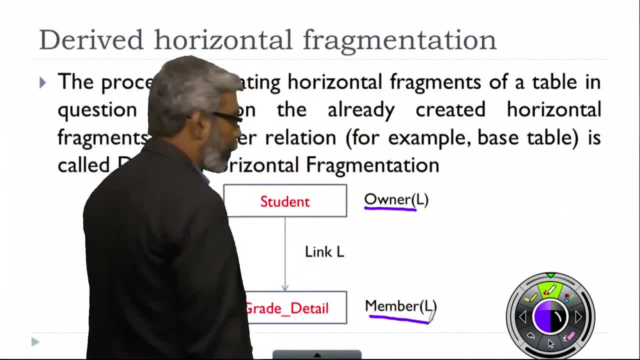 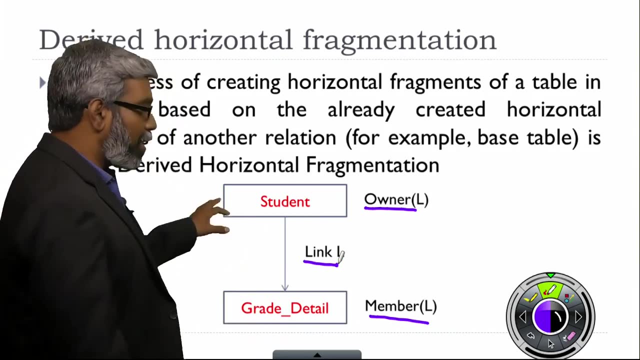 key as the owner relation, primary key as a owner relation and the foreign key table as the member relation. Now there is a link that connects these two tables. So we have the primary key in the owner relation and the foreign key in the member relation. Here 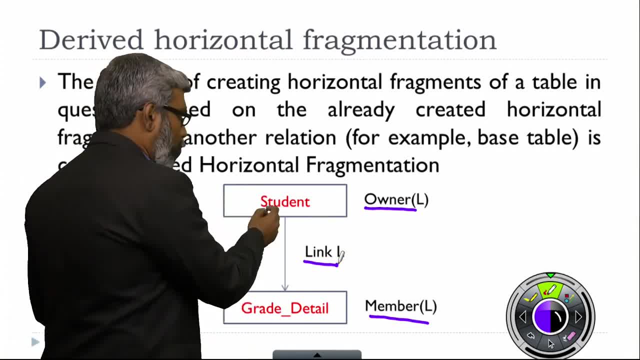 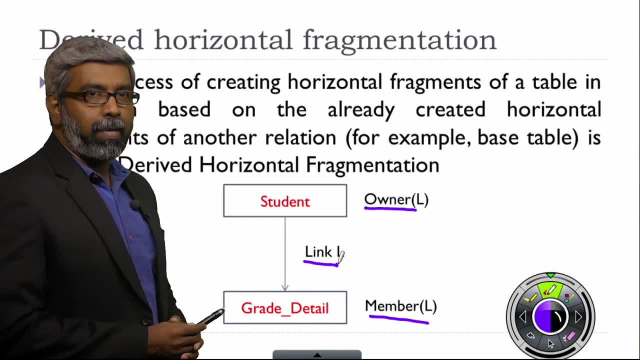 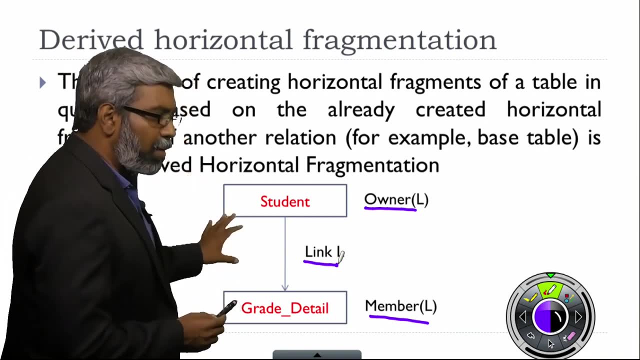 the domain of the primary key attribute of owner table and the foreign key attribute of member table are going to be same. So now the idea is I am going to fragment one of these tables using primary horizontal fragmentation And the additional directly which I did to get the Hi total of those primary and the 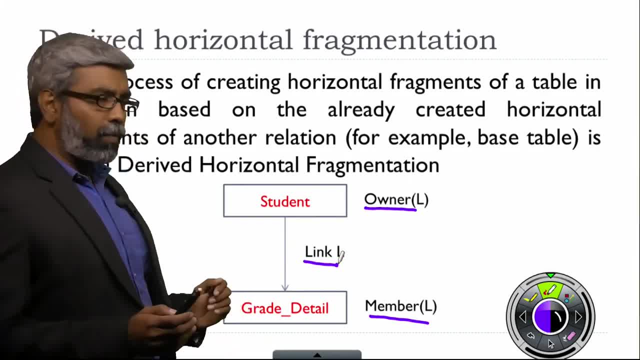 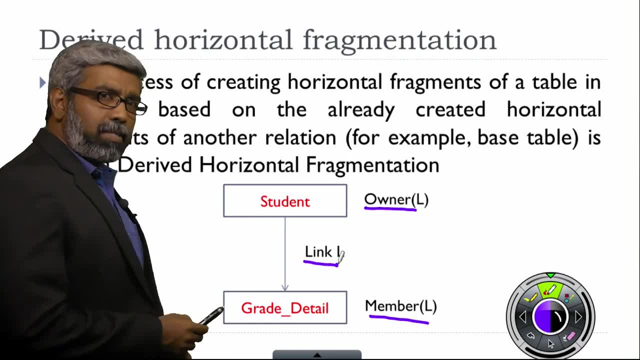 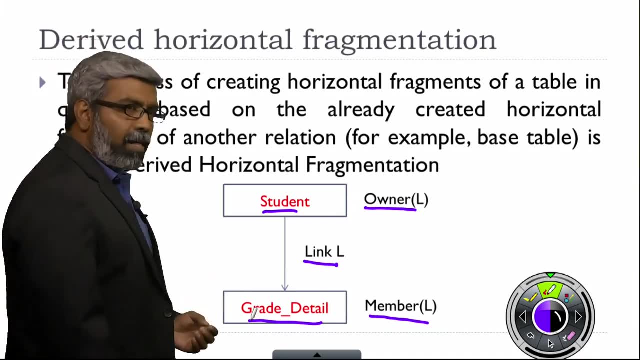 other one using derived horizontal fragmentation. So which is the table? So let us for example these two tables student. as well as the grade detail, both the tables are going to share an attribute which is common in domain, which is common in domain of permitted value: the 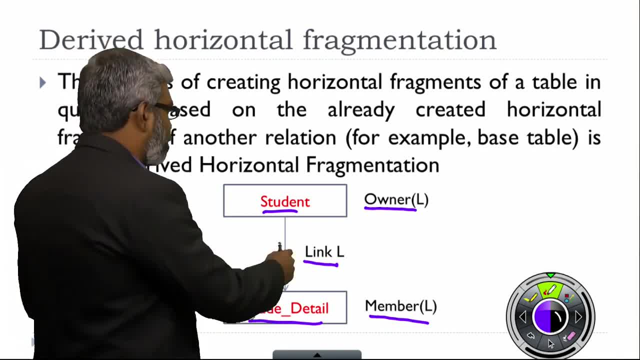 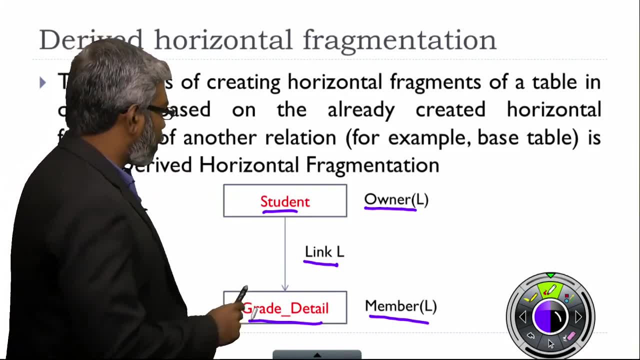 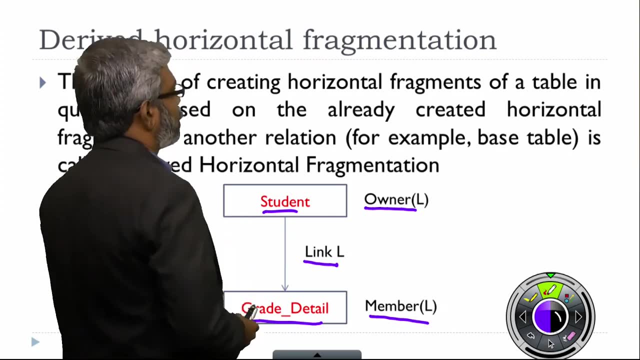 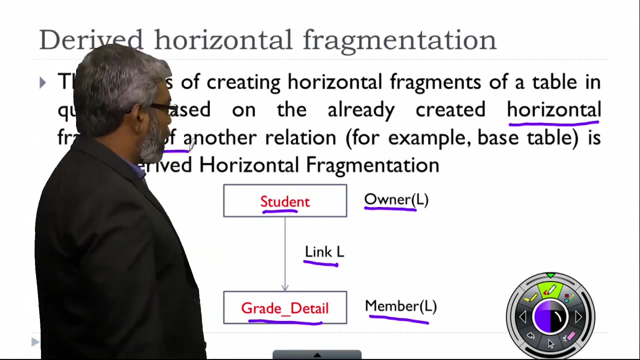 permitted value stored in these two tables. Now we take the primary table, that is, the table with the primary key, and we fragment the table using primary horizontal fragmentation. Then we use the fragments. we use the horizontal fragments that were created from the student relation, from the student relation. 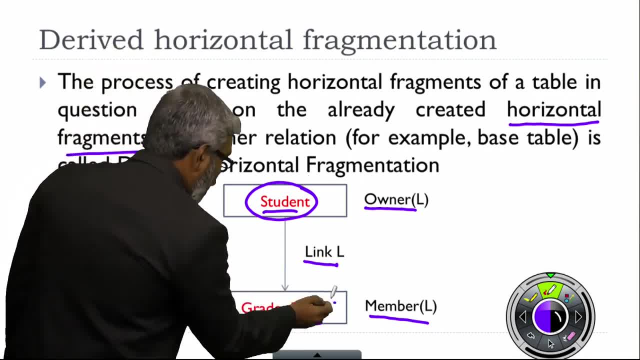 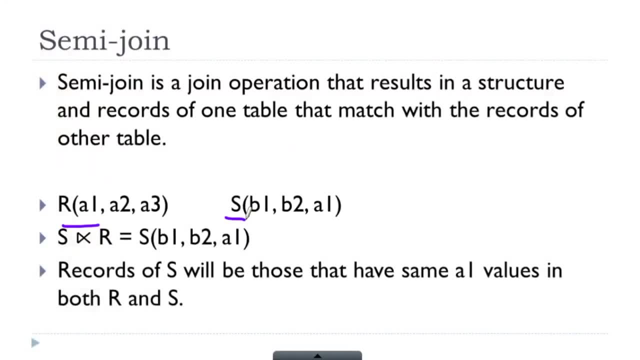 To further fragment the member relation, that is, in our case, the grade detail. Semi-joint is a joint operation that results in a structure and records of one table that match with the records of the other table. So here you see, we have two relations. one is R, the other 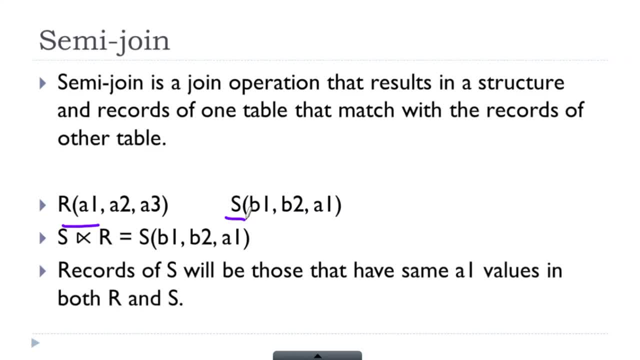 one is S. R has three attributes: A1, A2, A3,. S has three attributes: B1, B2, B3, B4,, B5, B6, B6, B7, B8, B9, B10, B11, B12, B12, B12, B13, B13,, B14, B14, B15, B15, B16,, B16,, B17,, B17,, B18, B19,. 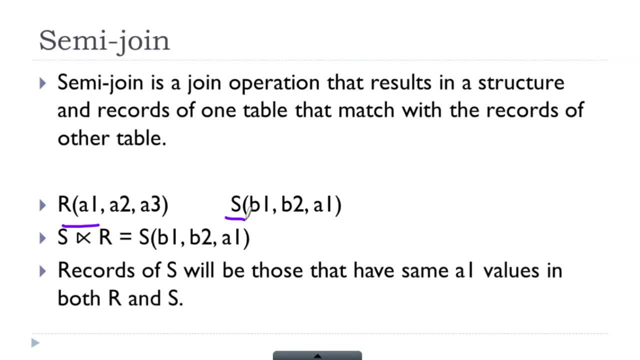 B19,, B12,, B14, B13.. S has three attributes: B1, B2 and A1.. If you observe this from these two tables, you can understand. A1 is the attribute which is common between these two tables. In many cases the name may be same or may be different, But the thing is the domain. 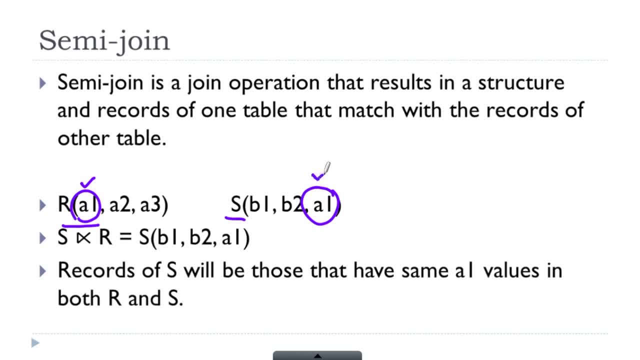 of this attribute and the domain of A1 in s. both are same. Now the symbol. this symbol is the semi-joint symbol, So S semi-joint R is equal to. I will get the structure of S alone. You observe carefully, See, it looks like S as it is, without any changes. So no. 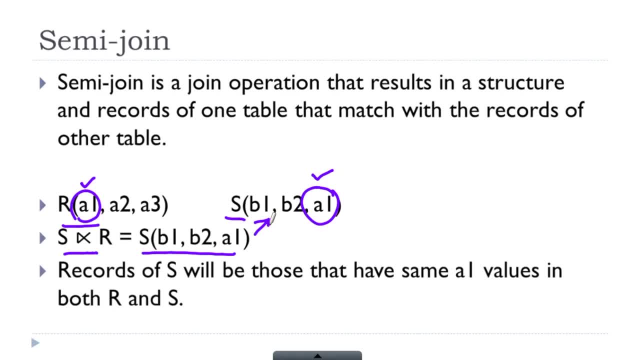 attribute is taken from the relation R, So this is semi-joint. But what about records? The records are filtered. Records are filtered on comparison of A1 of table S with A1 of table R. If both values are same, that record will be included in this fragment. So S semi-joint. 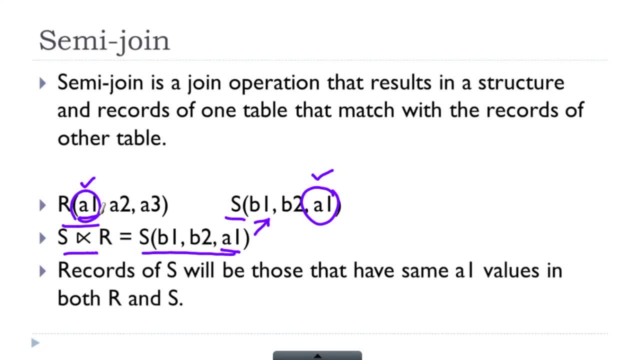 R see that the semi-joint it is open on the right hand side. That means we do not take attributes from the right hand side On the left hand side table. we take all attributes from left hand side table. So this results. 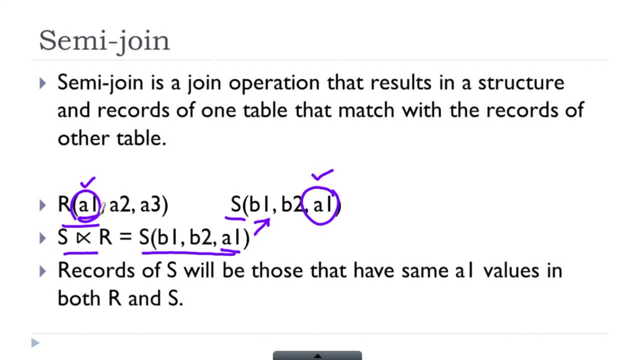 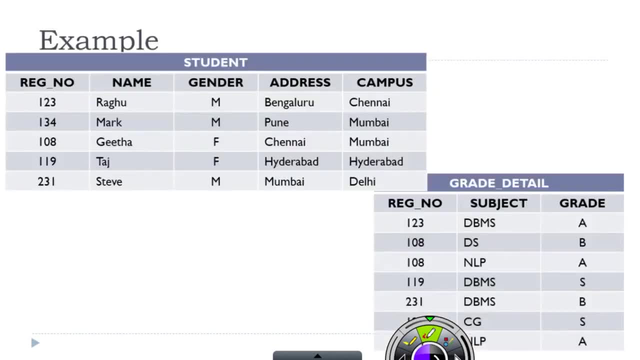 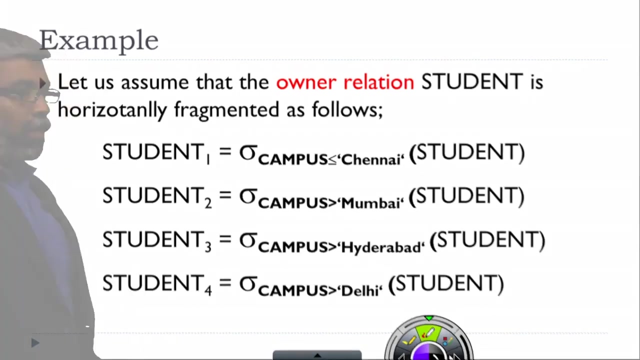 in records of S will be those that have same A1 values in both R and S. Now let us see an example, this table: We have student table with some records and we have grey tables with some records. Let us assume that the owner relations student is already horizontally fragmented horizontally. 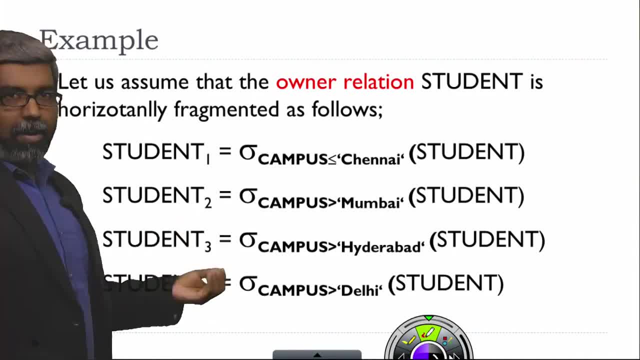 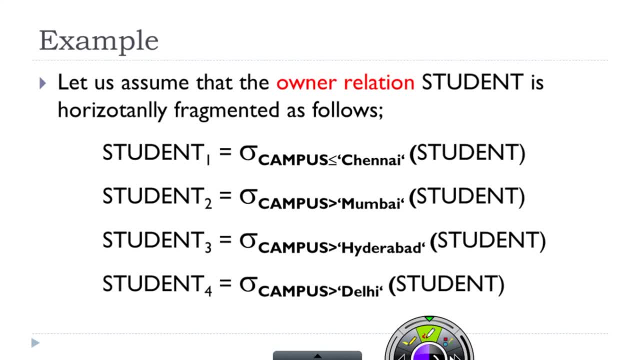 fragmented on the campus attribute of student relation and the values chosen are Chennai, Mumbai, Hyderabad and Delhi. That means we have 4 different sides at each of these locations because we have campuses in these locations. We have a campus in Chennai, we have a campus in Mumbai, Hyderabad and Delhi. That means 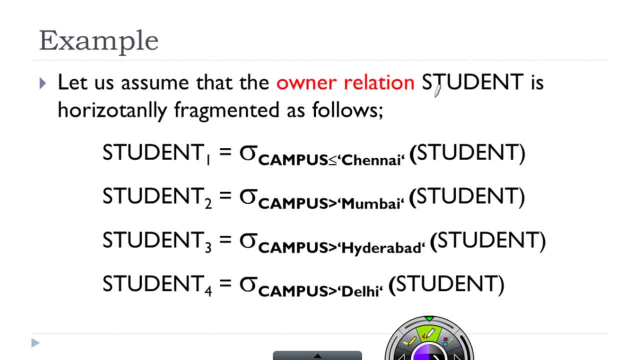 we have already assumed that we have already fragmented the student relation according to this fragment, that is, min term predicate and min term min term fragment value- campus Chennai. Now what we have is student 1, student 2, student 3 and student 4.. Now, if I am going, 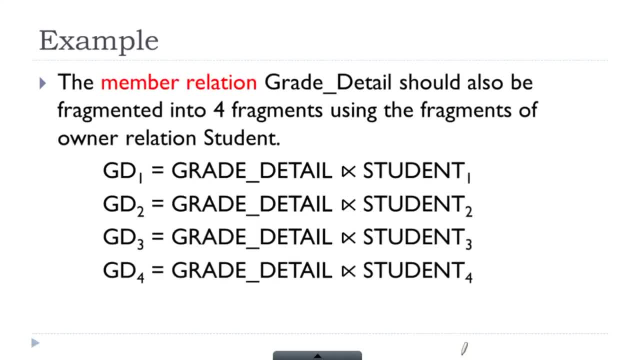 to join this table, the member relation, gray detail, should also be fragmented into 4 fragments only because the primary table, that is, primary key table, student, is already fragmented and into 4 fragments. So what we expect is we want to fragment the member relation in such 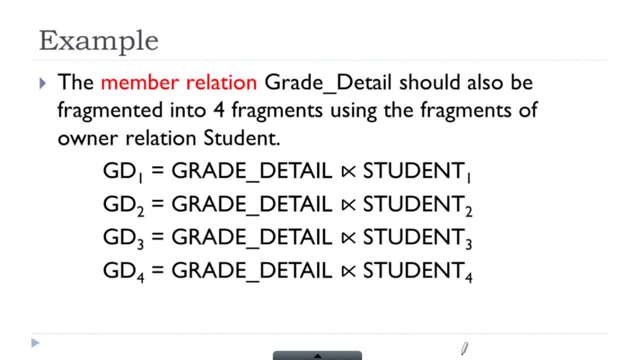 a way that the records related to those 4 already fragmented table will end up in the same fragment, that is, same site. So that is what we are applying: the semi-join operation. So how did you apply the semi-rejoin operation? So we create the gray detail 1, gray detail 1 by performing the semi-join. 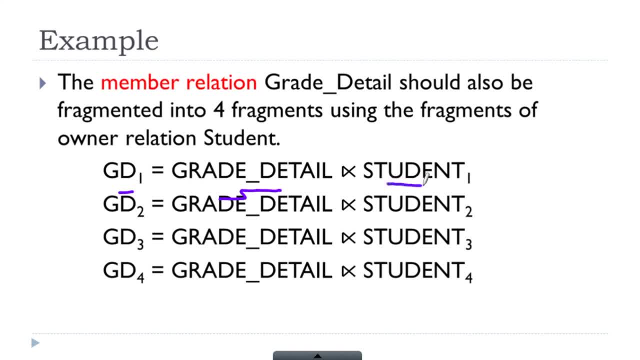 between gray detail and student table, student 1.. Student 1 is the fragment that is that was resulted from the applying the min term predicates, predicate 1.. Likewise, GD 2, the same gray detail table, is semi-join with student. So now what happens? 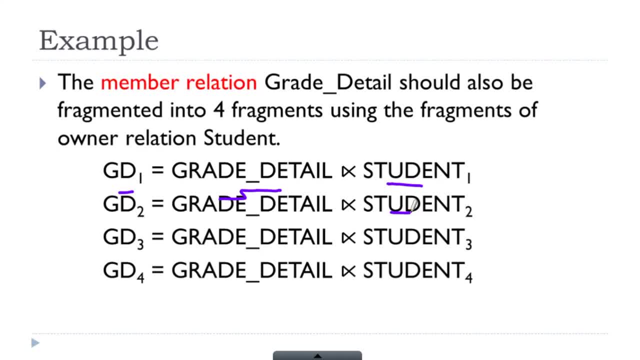 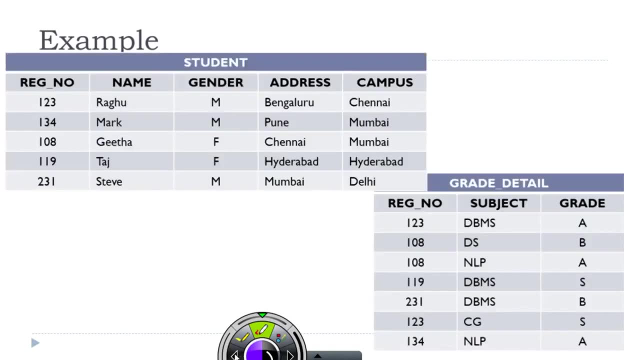 Student 1 have. assume that student 1 have 10 records. gray detail have all the records of it. Now the common attribute value, in our case the student register number, is matched with. see here. register number of the student is common in GD 2.. So the student register 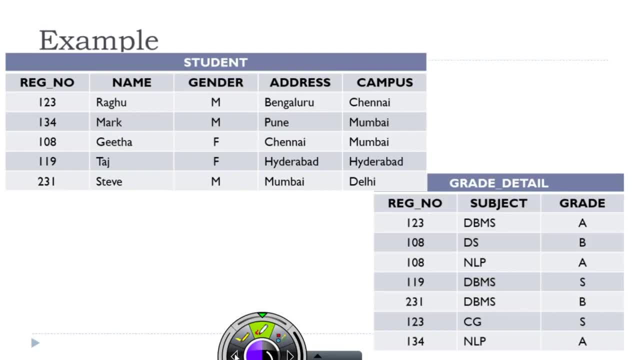 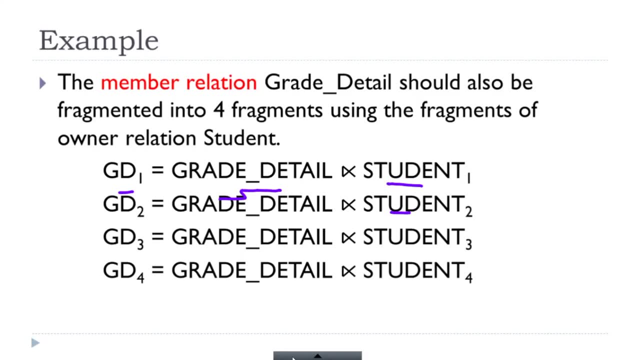 number of the student is common in GD 2.. So in our case the student register number is in both relations in student and gray detail and these two are compared. So the records of student 1 and gray details are compared on the value of the register number attribute. 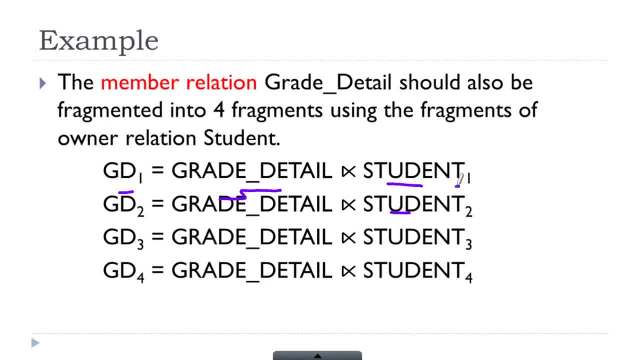 So only the register number of student 1 will match with the register number of the gray detail. So what we have- We have the fragment of gray detail- is according to the register number of student 1.. That is now student 1 and GD 1 will have the records of same person, same set of people, So that 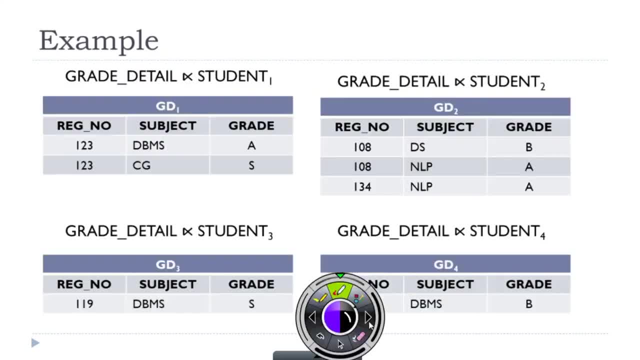 is the idea of this derived horizontal fragmentation. See example here. what did we do So? gray detail semi-join student 1, it is end up in 2 records, 2 records. Now the idea is the register number 1,, 2, 3 is the only student who end up in fragment 1.. Likewise in gray. 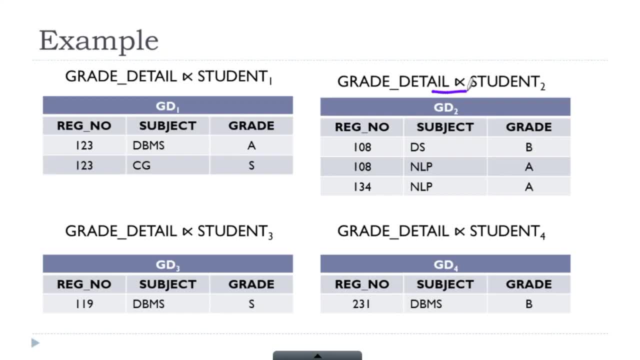 detail 2, there is gray detail 2, what we have is 108 and 134.. So these 2 students are part of student 2 fragment. Likewise, we have fragmented into 4 fragments, 4 fragments. Now the related details end up in same size. 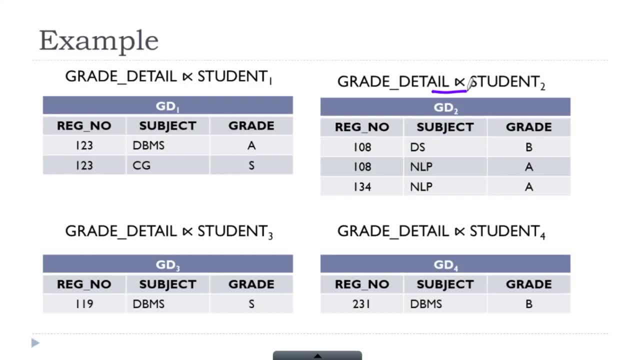 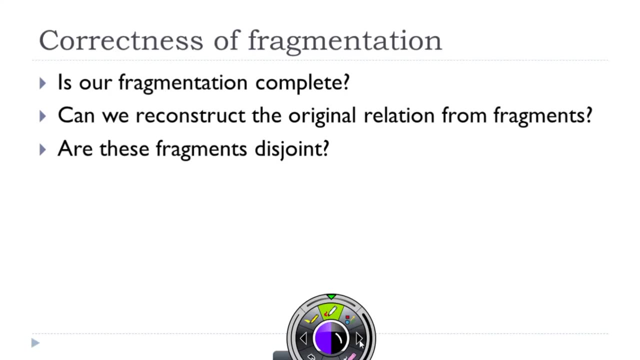 1., 2., 5.. So one particular site, all these records are end of thing. So this is what the derived horizontal fragmentation is about. So once we finish this one, there is an important step that is correctness of fragmentation. So this is very, very important, that is. 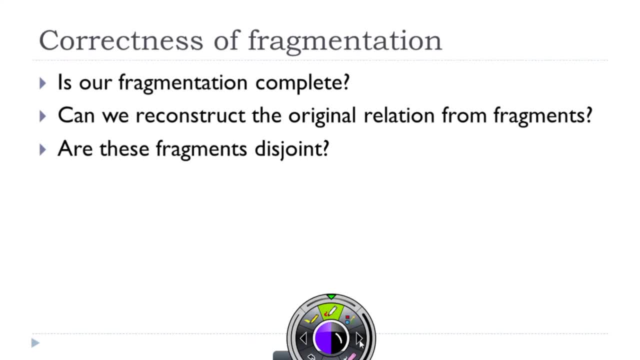 it is to check whether we have missed any data during fragmentation or any data is added extra, So that we want to be careful about this. So, correctness of fragmentation, the first one is: is our fragmentation is complete or not? So how do we check that? Are we missing? 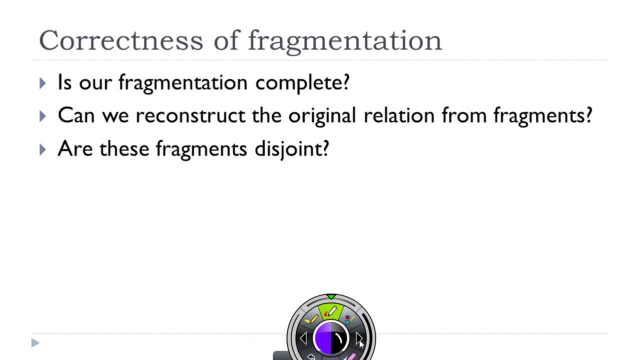 any data So that data should be available. that data of great detail should present in any one of these fragments. at least, it must be part of any one of these fragments. That is what the first rule is about. The second rule: can we reconstruct the original? 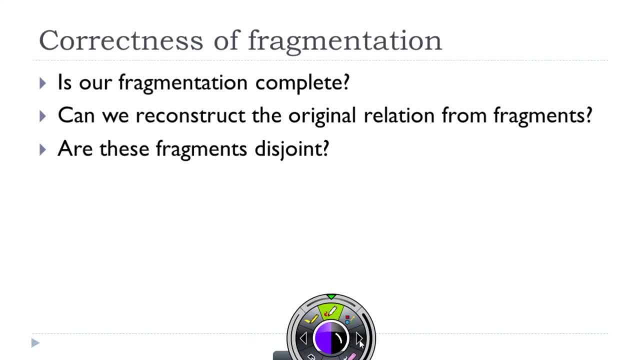 relation from fragments. That is, I perform joining of, that is, union of all these fragments and I will end up in the original great detail table. And the third condition is: are these fragments disjoint? So disjoint is a property that ensures there is no redundancy exist. 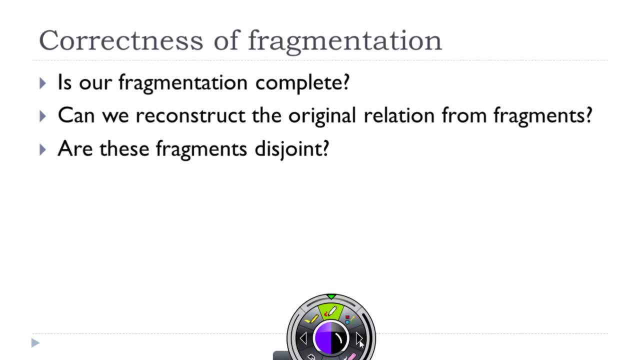 in a while fragmenting the relation. While fragmenting the relation, we want to be careful about no record should be part of more than one fragment. So, that is, we want to find all these fragments or disjoint. So if you perform intersection between all these table, 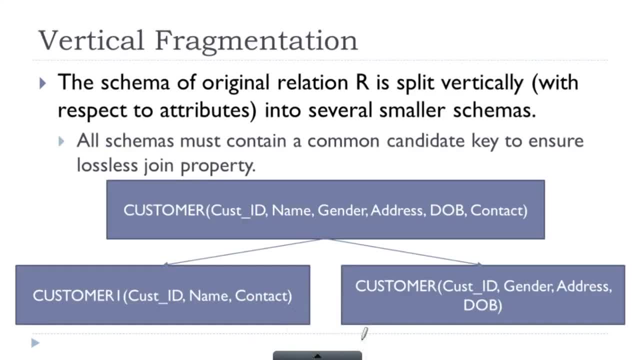 we will end up in no record for disjoint. So this is the first rule. So this is the first rule. So this is common Vertical fragmentation. the next concept is vertical fragmentation. So I already we have finished with the horizontal fragmentation where we have discussed about 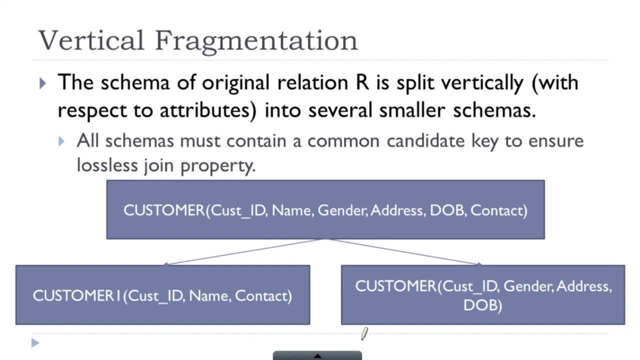 two varieties. one is about primary horizontal fragmentation. the other one is about derived horizontal fragmentation. Now, the next one is vertical fragmentation. So we are going to discuss about a little bit about vertical fragmentation, not too much about this. So vertical fragmentation is a way of decomposing a table, So this: 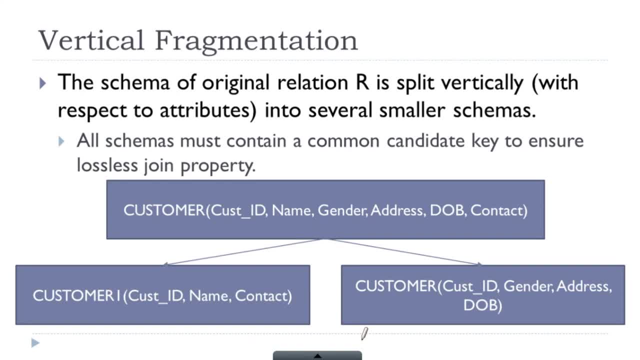 is a way of decomposing a table into two or more tables, A simple way of decomposing a table into two or more tables. Why do you want to do that? In some cases we have a big table, the big table, not all the columns of these big tables, not all the 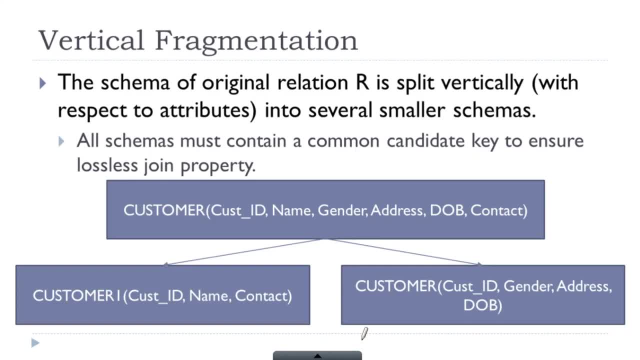 attributes of this big table is needed in all the different sites that we have in a distributed database system. We may have something like one portion of a table. one portion of of this table is interested in all the sites. one portion may be very much interested to. 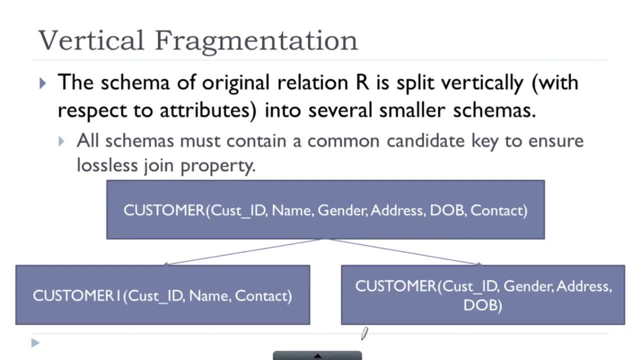 only one particular site. That is. in such case, I want to fragment my table vertically so that I can place the part which is common for all in one location, which is unique for each site, at each different sites. That is what we want to do. That is why we use vertical. 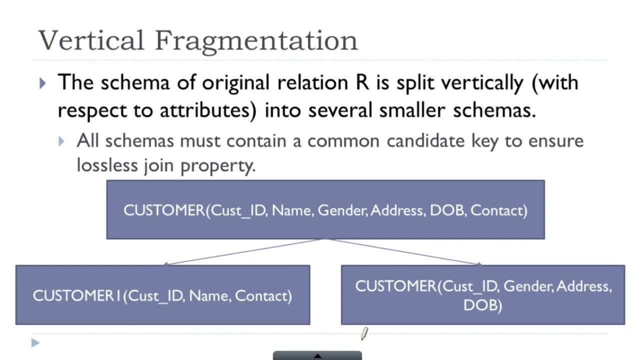 fragmentation and it is just like the process of vertical fragmentation. it is decomposition. decomposition, that is, during the normalization process you must have studied decomposing a relation into two or more relations. So the schema of original relation R, that is, a structure of relation R, is split vertically. 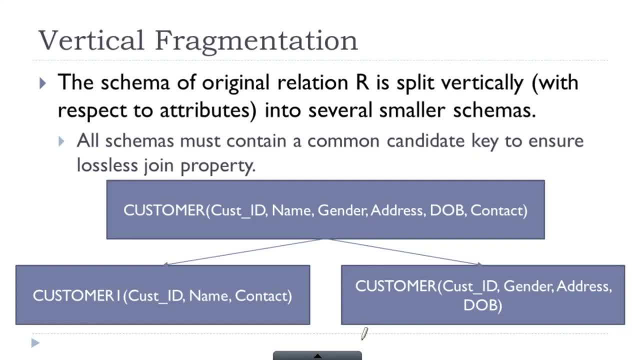 vertically, With respect to attributes, into several smaller schemas. Now, all schemas, one property is. all schemas must contain a common candidate key to ensure lossless joint property. Lossless joint property. what is that? So during the decomposition, we are going to break a table. 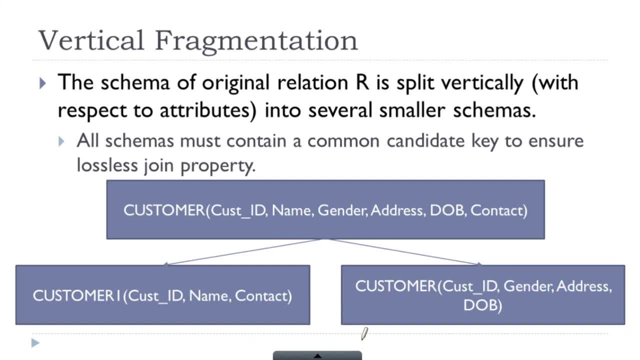 in such way that we want to retain the losslessness property. The reason why I break my table is to use it differently. So the ways are: I may use the fragment, that is, one fragment alone, or I want to join these 2 relations back to get. 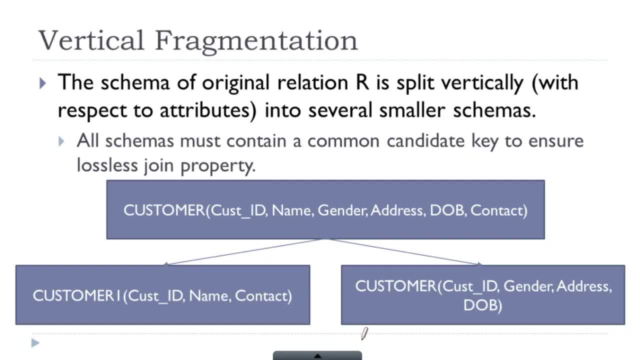 the original relations output. So there are different requirements, So that we must ensure the lossless joint property. That means I broke my relation into two or more relations. So perform join between, join operation between these fragmented relation. I must end up in. 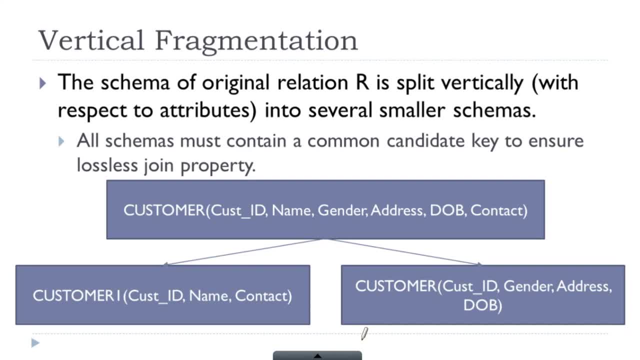 original relation without losing any information- any information. That is what the lossless join property is all about. See an example here. there is a customer relation with a schema: customer ID, name, gender, address, DOB and contact. Now we want to fragment this relation vertically. that means 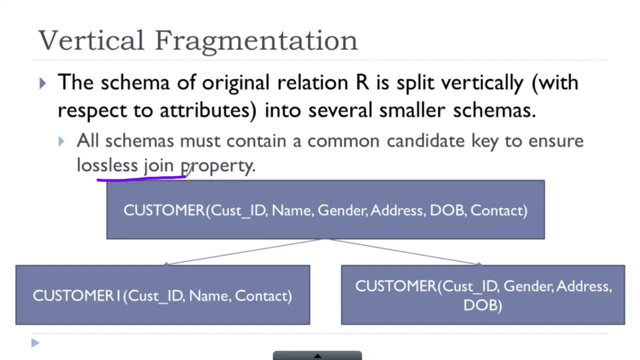 customer ID attribute, name attribute, contact attribute into one fragment and in another fragment custom gender address and DOB. gender address and DOB we want to break into into separate relation. The reason would be like this: gender address and DOB may not be frequently. 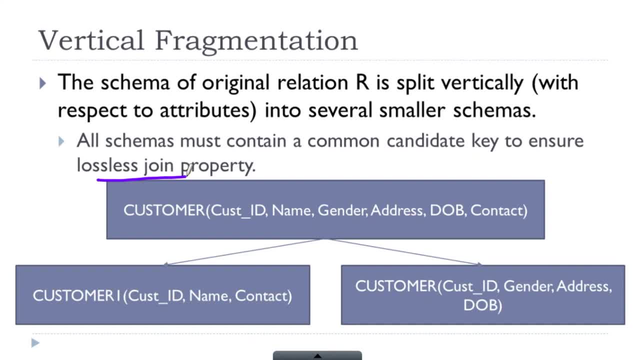 accessed by the application. On the other hand, customer ID, name and contact may be accessed frequently So that we want to place it in In different locations according to our requirement. application requirement. Now, when I break this table, I cannot get the original relations back, So what is necessary is there should. 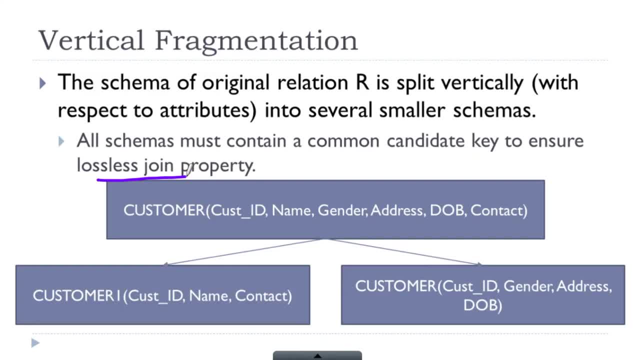 be a common candidate, common candidate key. So what we have is here the customer ID is taken, which is the primary key of the table. This table is taken into both the fragmented relations. Now what we have is the vertical fragmentation of the relation customer. And if suppose this, 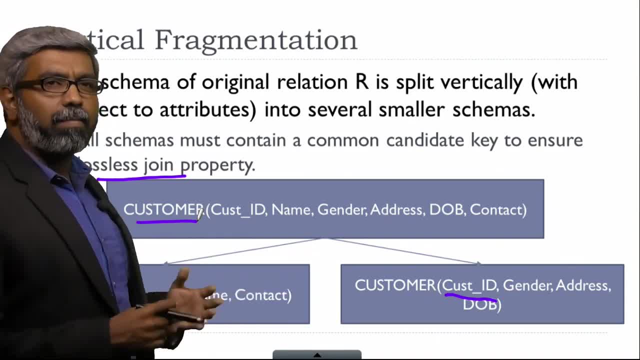 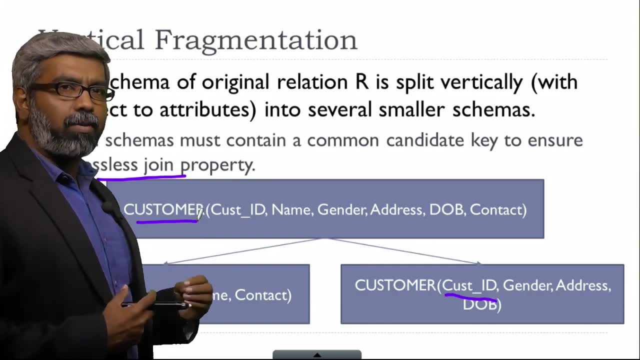 is. this is very simple way of doing this one. I just want to break my relations to two or more relations, And it is based on the applications that are trying to access frequently. This portion may be accessed frequently. Customer 1 may be accessed frequently, or the customer. 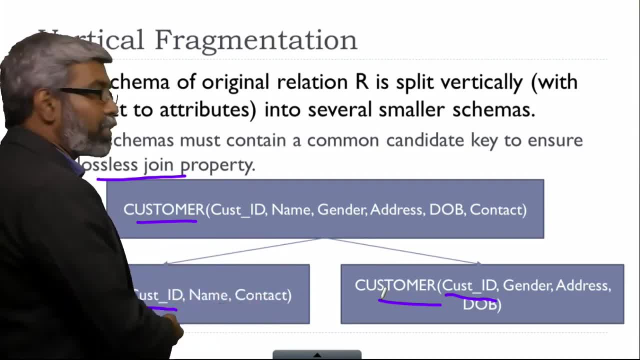 2 may be accessed frequently. So this is a very simple way of doing this one. So this is a very simple way of doing this one. So this is a very simple way of doing this one. Customer 1 is accessing frequently in different locations- not in the same site, in different. 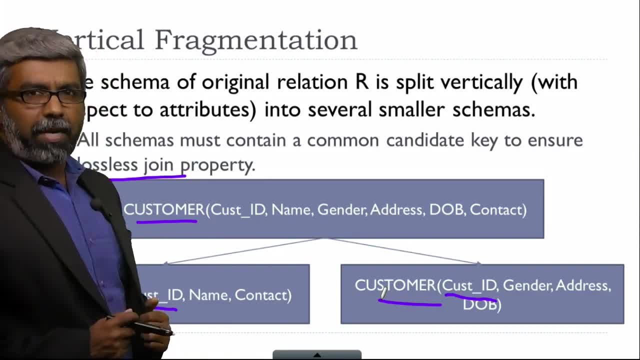 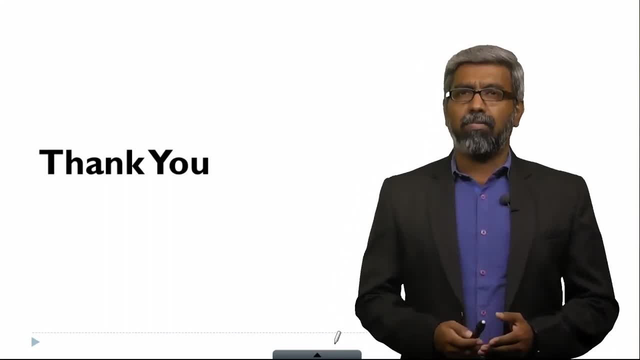 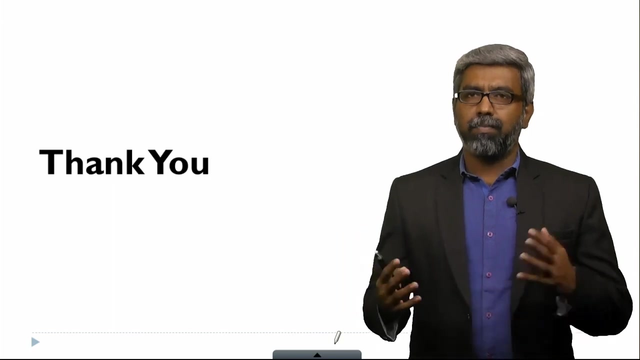 sites. So accordingly, we are going to fragment the relation vertically. We have discussed about derived horizontal fragmentation. The purpose of derived horizontal fragmentation is to fragment the entire database and we want to break other relations with respect to already fragmented tables. So every other table is already fragmented And every other table is already fragmented.